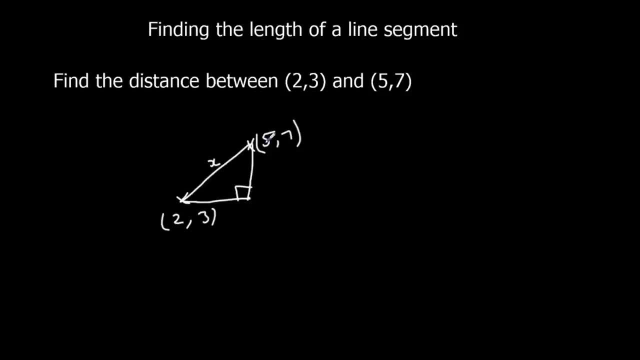 and use Pythagoras for this. So between 2 and 5,. how far have we gone along the x? So between 2 and 5,. how far have we gone? We've gone 3 along. 2 to 5 is 3, and from 3 to 7,. 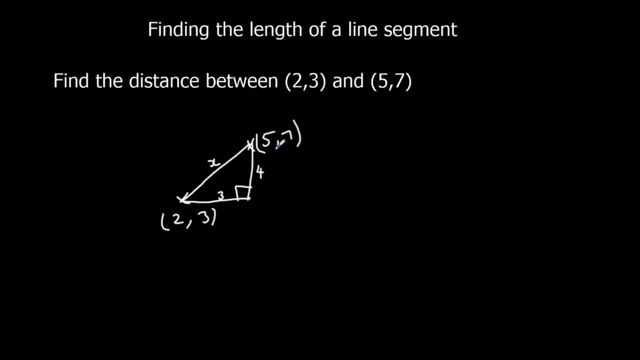 that's 4, right Up. So we've gone 3 along and 4 up, And then we just do Pythagoras. So a squared plus b squared equals c squared. So 3 squared plus 4 squared is x squared. 9 plus 16 is x squared. 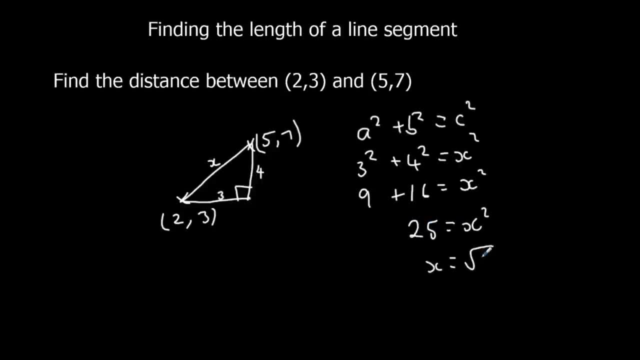 25 is x squared. x is the square root of 25, which is 5.. So the distance between these 2 points is 5.. So if we do the same thing again, it doesn't matter if it's going to go down In this case. 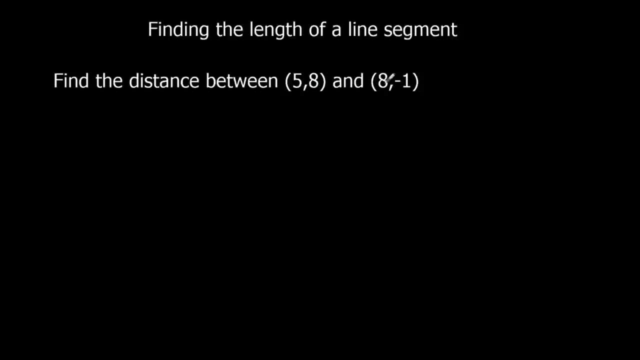 it is. The only thing that really matters is the distance between the x's and the distance between the y's. So I'll draw it accurately, if I can. So 5, 8 here, and then along to 8 minus 1.. So let's go there. So it's going to go, it's going to go down. 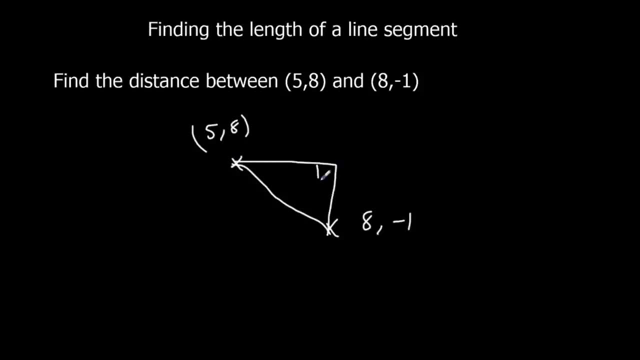 this time, But that doesn't really matter. So 5 to 8, how far have we gone along the x? 5 to 8, that's 3.. 8 to minus 1, that's a difference of 9.. It's gone down 9.. So 9 and x, And then it's just. 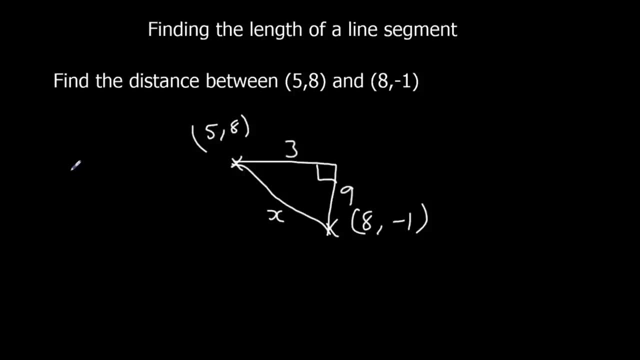 a Pythagoras question again. So a squared plus b squared equals c squared. 3 squared plus 9 squared is x squared. 9 plus 81 is x squared. So 90 is x squared And x is the square root of 90.. We'll leave it. 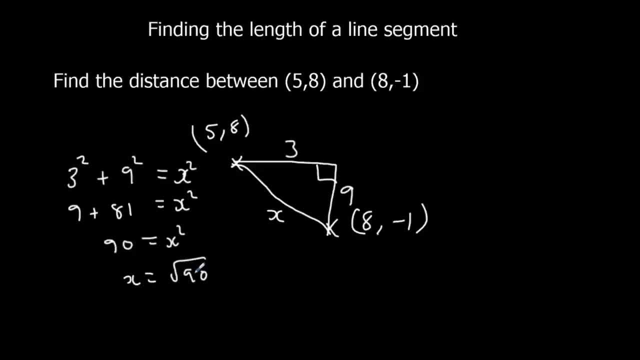 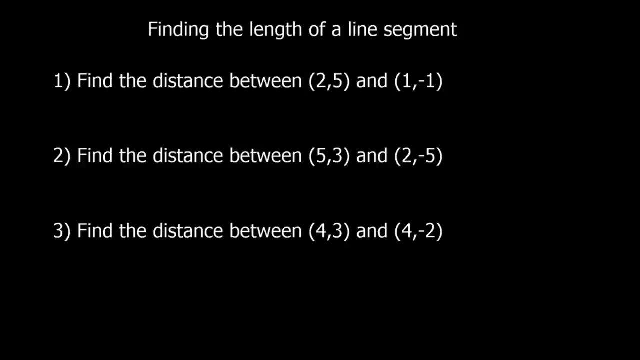 we'll leave it as a square root of 90 before for now. sorry, This will simplify into well, 3 root 10.. But we'll leave it. Square root 90 is fine. Square root 90. Okay.